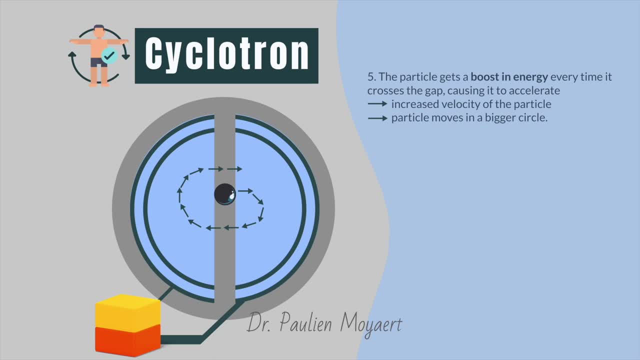 and this in turn will force the particle to move in a bigger circle. After another half rotation the electric field in the region must be changed again so that the charged particle can be accelerated again. So we use an alternating electric field where the frequency of the voltage is set so that 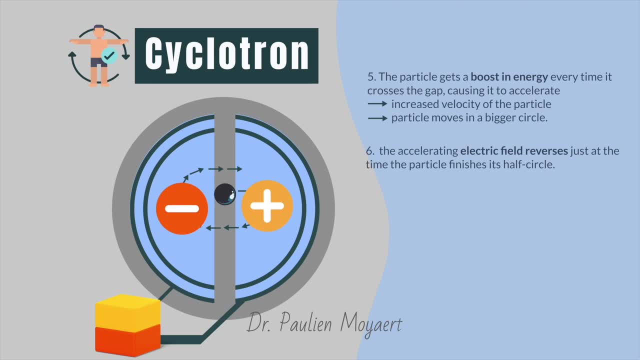 the particle makes one revolution during a single cycle of the voltage. In other words, the accelerating electric field reverses just at the time the particle finishes its half circle. After repeating this process several times, the radius of the high speed particle reaches the radius of the cyclotron. 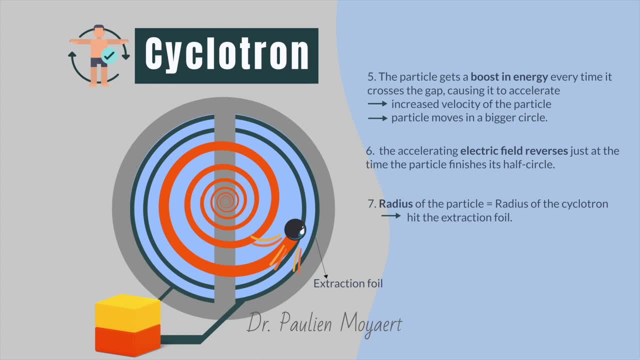 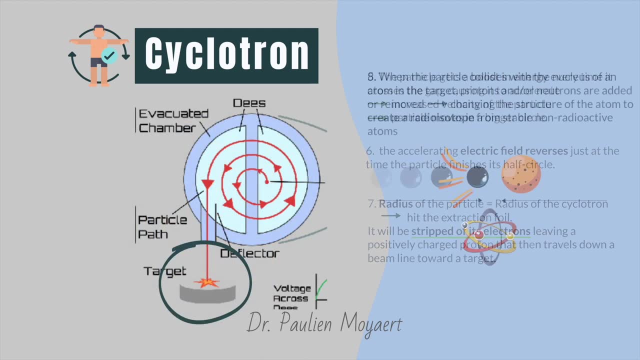 The particle will hit the extraction foil and it will be stripped of its electrons, leaving a positively charged proton that then travels down a beamline toward the target. When the high energy particle collides with the nucleus of an atom in the target, protons 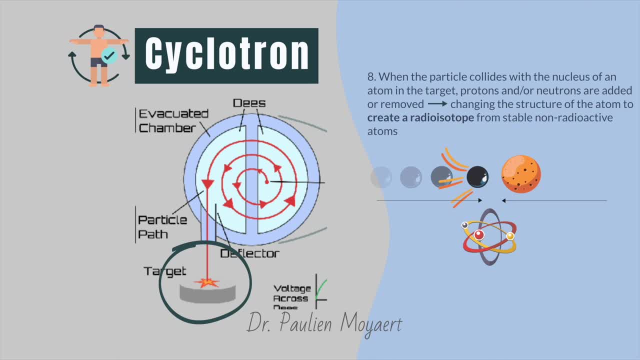 and or neutrons are added or removed, thereby changing the structure of the atom to create a radioisotope from stable, non-radioactive atoms. The radioisotope is then added to a molecule. For example, if we want to make FDG, we have. 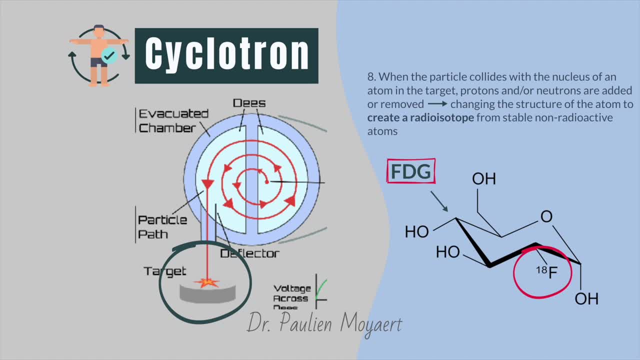 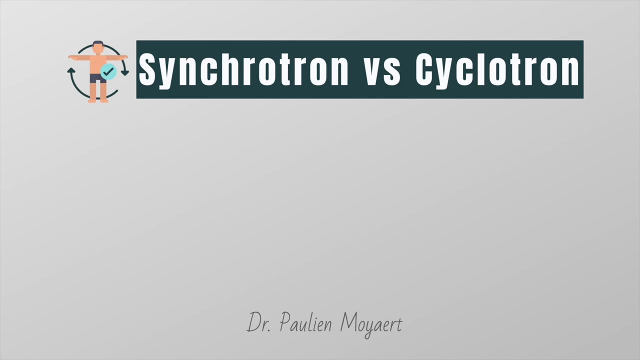 to produce fluorine-18 and incorporate this into a sugar molecule. Bombarding oxygen-18 with hydrogen ions results in the production of fluorine-18 and a neutron. One more thing I'd like to share with you is the difference between a synchrotron and 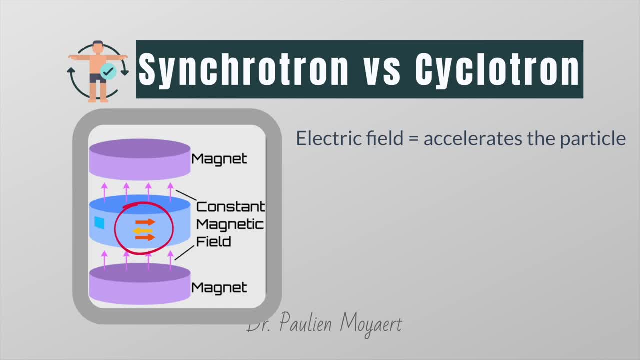 a cyclotron. Remember that the electric field creates a force in a charged particle and, as such, accelerates the particle. The magnetic field, on the other hand, constrains the charged particle to circular or spiral orbits, As the particle accelerates under the electric. 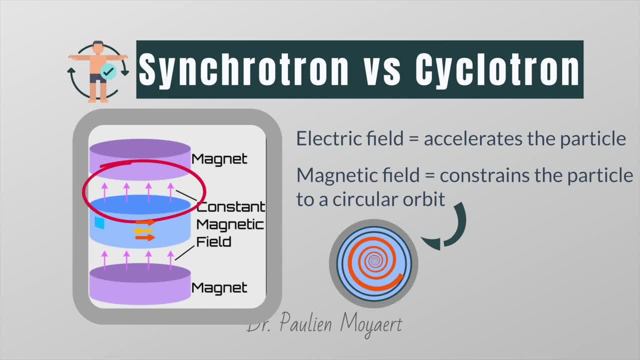 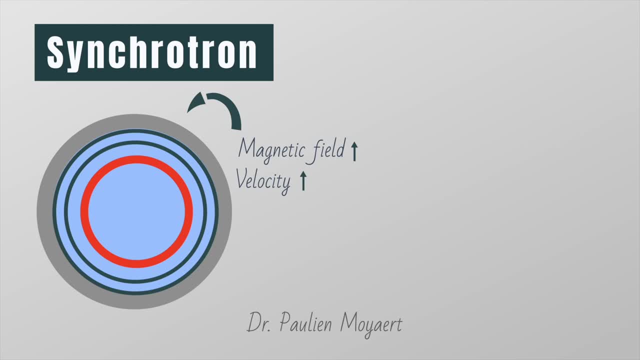 field. its velocity increases, causing it to move to a path of increased radius. To combat this, the magnetic field is increased to keep it constrained to circular orbits. This requires the magnetic field to be kept in synchronicity with the increased velocity. This is what happens in the synchrotron.